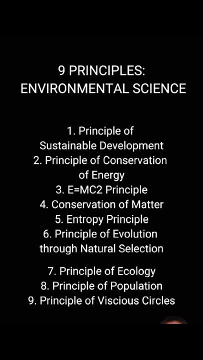 Environmental science has nine principles, namely as follows: 1. Principles of Sustainable Development. 2. Conservation of Energy. 3. Principles of Energy Equals to Mass Times, Speed of Life Squared. 4. Principles of Conservation of Water. 5. Principles of Entropy. 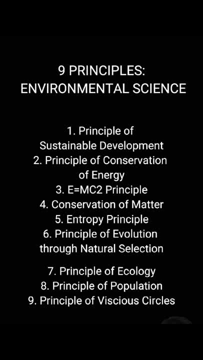 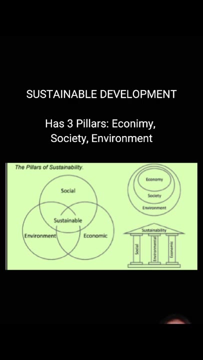 6. Principles of Evolution Through Natural Selection. 7. Principles of Ecology, 8. Principles of Population. 9. Principles of Vicious Service. The first principle states that we must move. We must move towards the adaption of a lifestyle that we maintain independently. 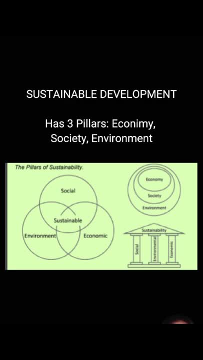 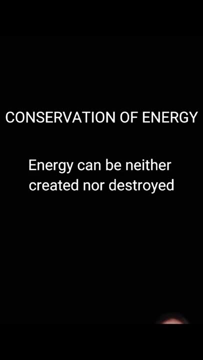 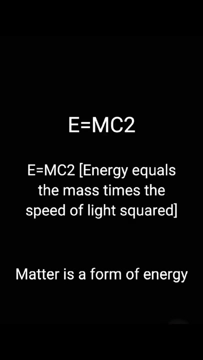 It means that we must stop destroying the very necessities of our very existence. The second principle is the first law of thermodynamics. This means that the quantity of energy is constant. The third principle is: energy equals to the mass times the speed of light squared. 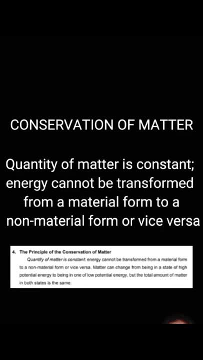 The fourth principle means the quantity of matter is constant. Energy cannot be transformed from the ground, From material to a non-material, then vice versa. It will be as if humans cannot use fossil fuels, uranium and metals, when the amount of usable energy needed to extract can exceed the amount of usable energy that we need to die. 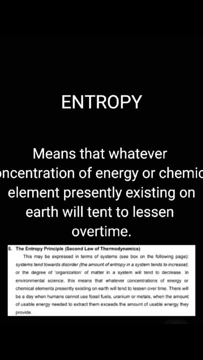 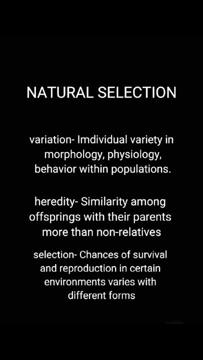 My use is yours: tripping on skies sipping waterfalls. My use is yours: run away now and forever. Life forms and earth have evolved from a common source. Each of the surviving of the species is a result of its genetically adapted based biology. 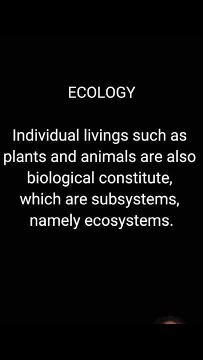 The next principle states that the system in which the human species interact are the physical and biological. The entropy law is against this principle. This means that living systems must exist and larger physical systems in which the total entropy is increased. The principle of population states that non-human population tends to increase and decrease. 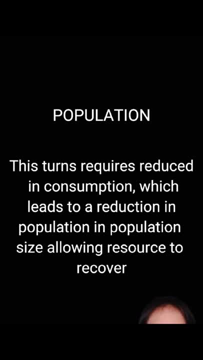 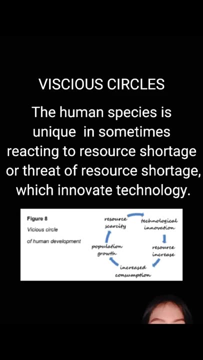 in cycles: The greater the number of species, the greater the food consumption, ultimately leading to the population's experiences of scarcity. The last principle of environmental science states that human development consists in an exhilarating movement from creation of resources to scarcity, to technology's innovation. 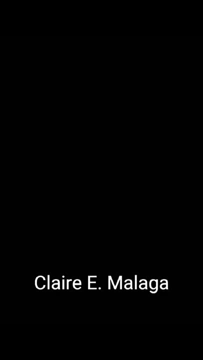 My use is yours: tripping on skies sipping waterfalls. My use is yours: tripping on skies sipping waterfalls.